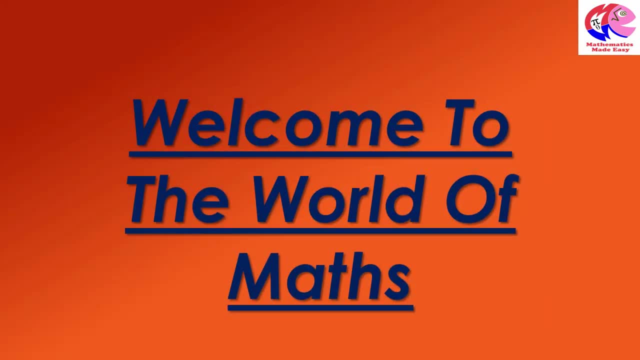 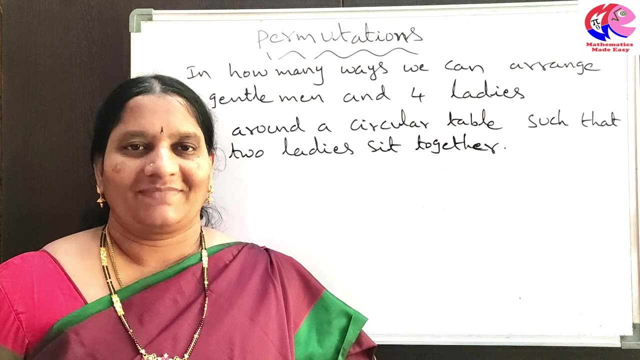 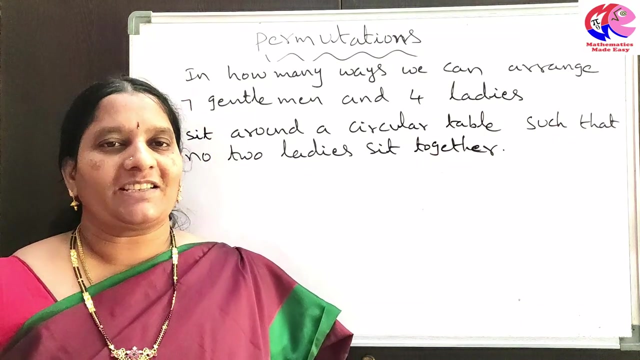 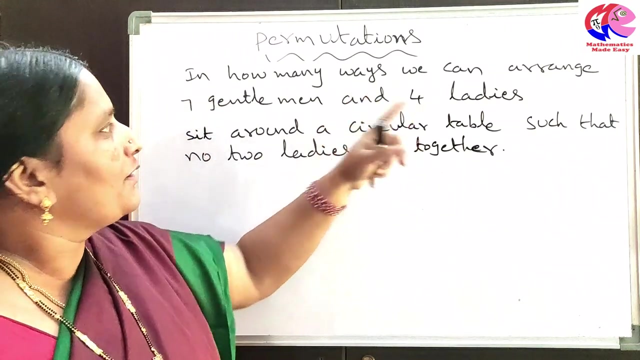 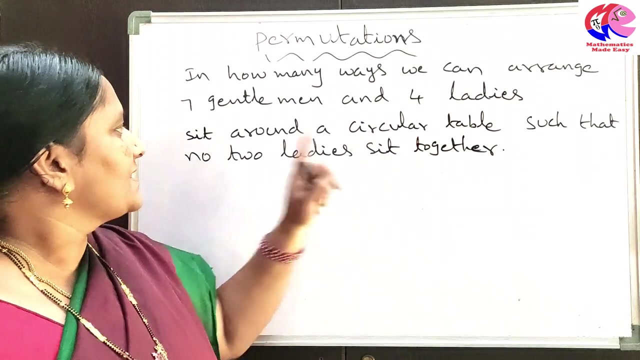 Hello everybody, welcome back to another session of Mathematics Made Easy. Now the topic is permutations. that too, it is related to circular permutations. There in the circular permutations, the question is in how many ways we can arrange 7 gentlemen and 4 ladies sit around a circular table such that no 2 ladies sit together. 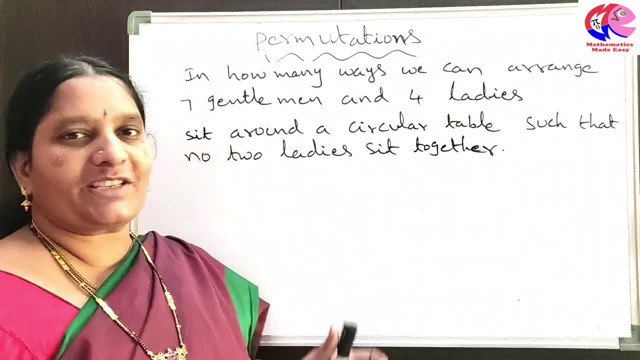 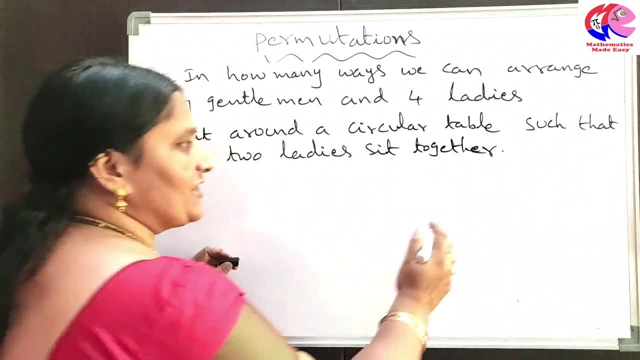 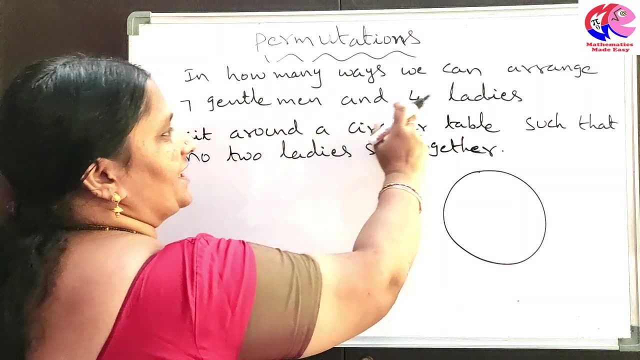 7 gentlemen and 4 ladies are sitting around a circular table and the condition is: no 2 ladies sit together. So first, let us arrange. let us take this is the circular table. Around this circular table we are going to arrange 7 gentlemen and 4 ladies. 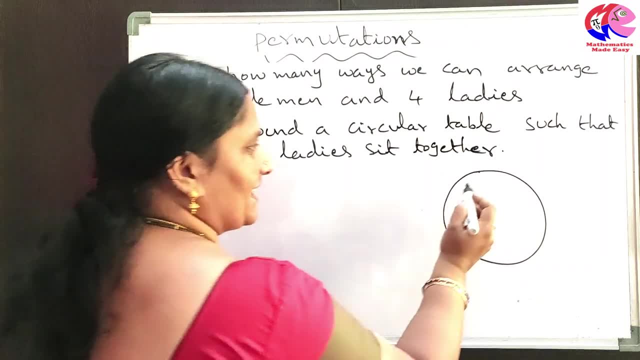 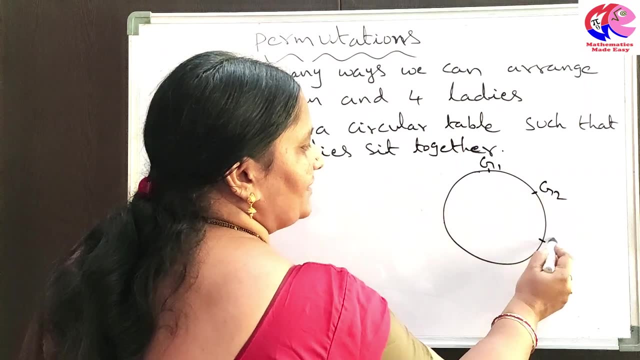 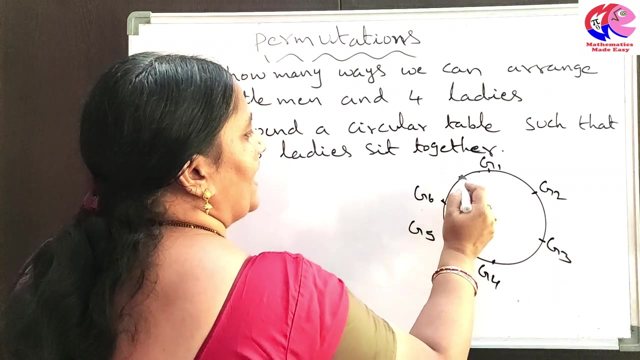 and the condition is: no 2 ladies sit together. First. let us arrange 7 gentlemen. here, then it is G1, let us take G2, G3, G4, and here it is G5,, this is G6, and here it is G7. 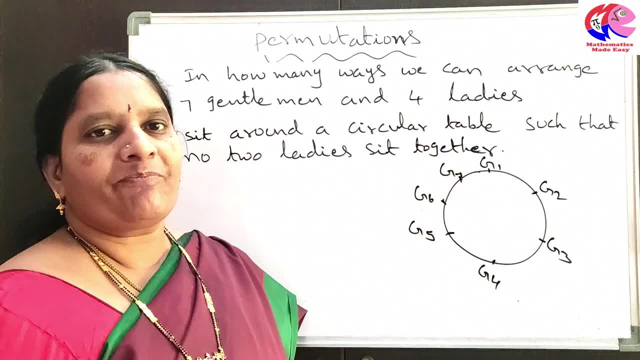 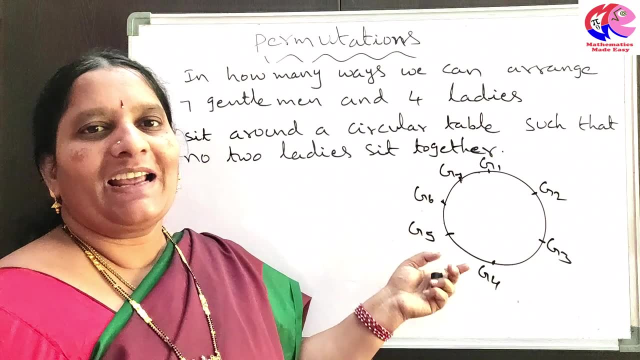 So 7 gentlemen, we can arrange around a circular table like this. Whenever we are arranging living things around a circular table, the condition is formula for finding number of circular permutations is formula for finding number of circular permutations is equal to n minus 1 factorial. 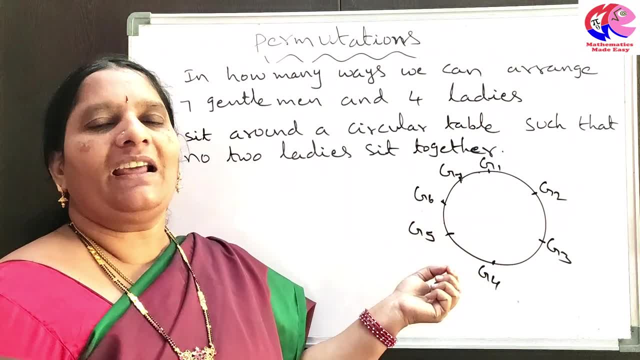 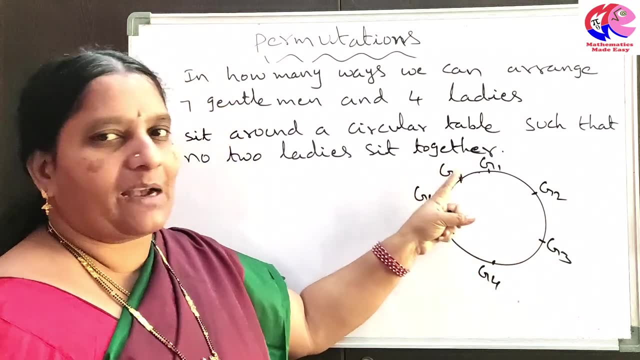 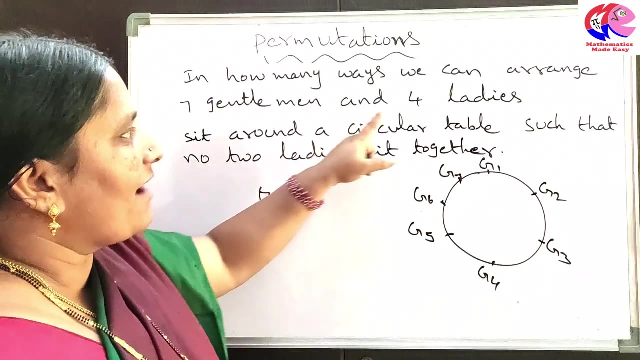 Whenever we are arranging living things around a circular table, formula for finding number of circular permutations is equal to n minus 1 factorial. So we can arrange these 7 gentlemen around a circular table in 7 minus 1 factorial ways, and we have to arrange these 4 ladies in the gaps. 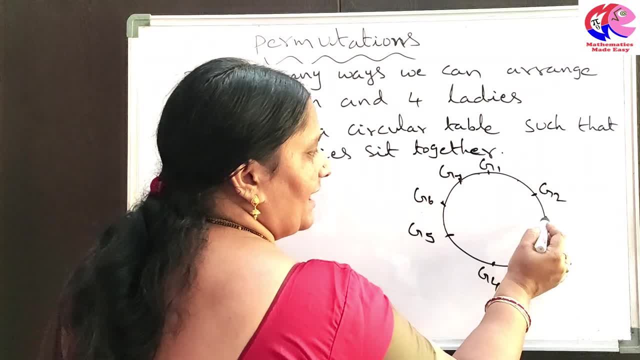 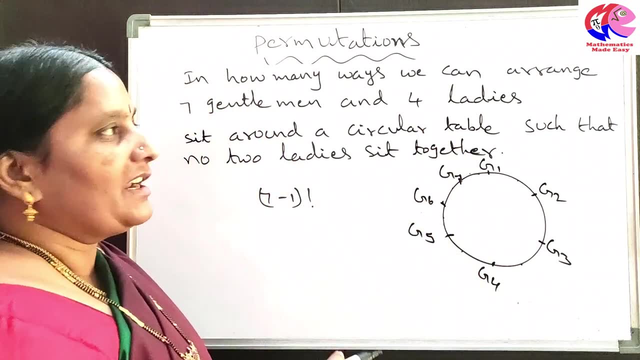 Now gaps are how many? let us check. This is gap 1, gap 2, 3, 4,, 5, 6, 7.. 7 gaps are there. 4 ladies are there. We can arrange 4 ladies in 7 gaps. in how many ways? 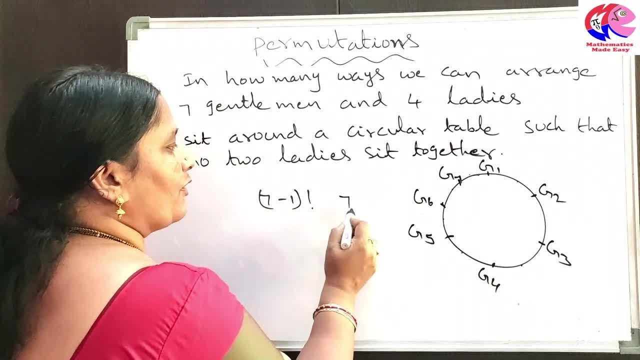 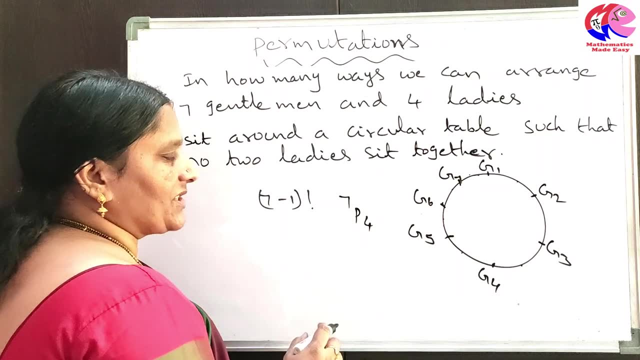 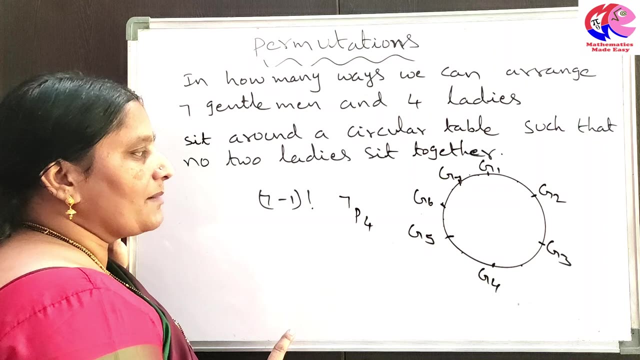 In MPR ways like that, In 7P4 ways, we can arrange these 4 ladies there in the 7 gaps According to principle of succession. if first work can be done in M ways, then total number of ways for completing the work is equal to MN MN ways.